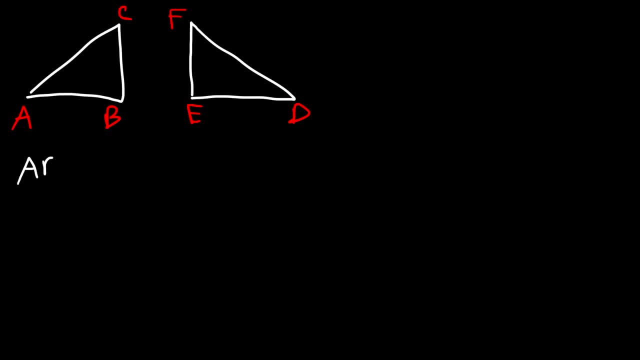 Now you're given that AB is congruent to DEF and also BC is congruent to DEF, BC is congruent to EF And that CA is congruent to FD. So your task is to prove that CA, or rather, 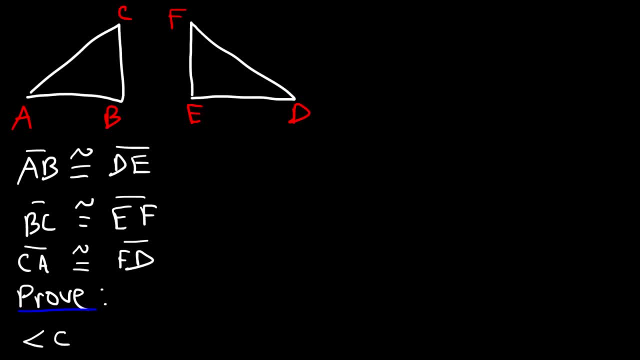 let's change it. Go ahead and prove that angle C is congruent to angle F. So let's make our two column proof Statements and reasons. So the first statement that we could say is that AB is congruent to DE. 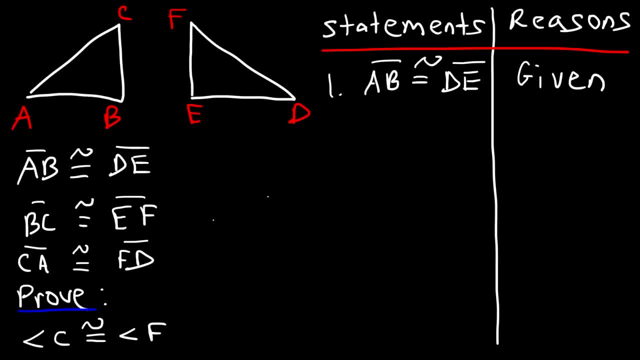 And the reason for that: it's given. So let's write that on the picture. So this is: AB is congruent to DE. Now in step two, we could say that BC is congruent to EF, And that's given as well. 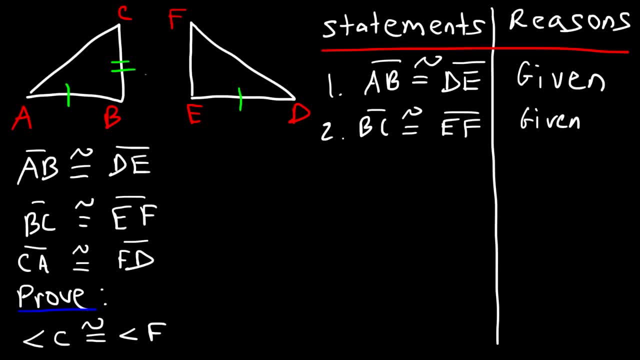 So here's BC, and it's congruent to EF. Now in step three, we could say that CA is congruent to FD, And that's also given. So now, what postulate can we use to prove that these two triangles are congruent? 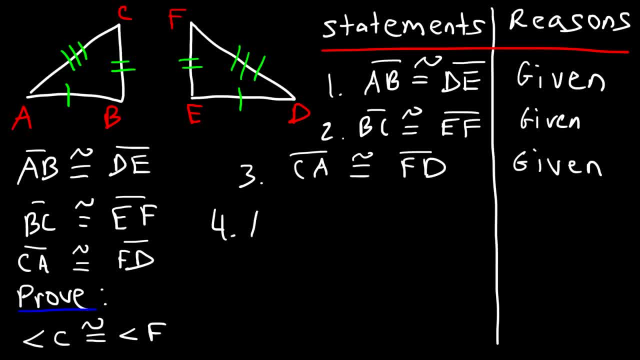 So in step four we could say that triangle A, BC is congruent to triangle DEF. Now make sure you write this in a certain order. Notice that A corresponds to BC And D corresponds to EF And BC is equal to EF. 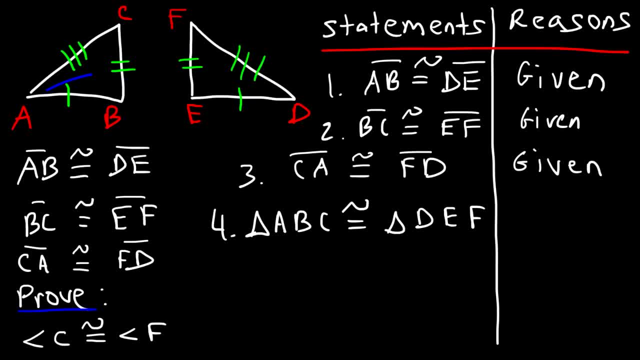 based on the two tick marks that you see there. So A has to match up with D. B is opposite to the side with three tick marks. The same is true with E. So when saying two triangles are congruent, B has to match up with E. 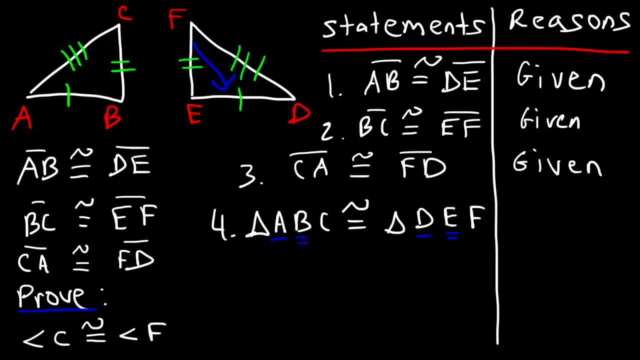 F is across the side with one tick mark and C is across the side with one tick mark. So C and F correspond to each other. So for those of you who might be wondering how you should write these letters and in which order, 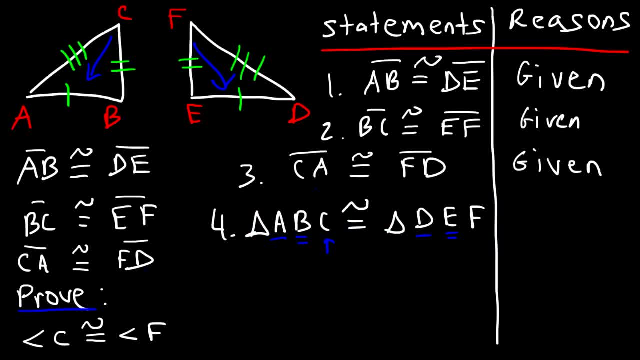 make sure that the first two angles match up. Angle A has to be congruent to D And typically, if the sides are congruent, then the angles opposite to those sides has to be congruent, based on the side angle theorem. Now we can. 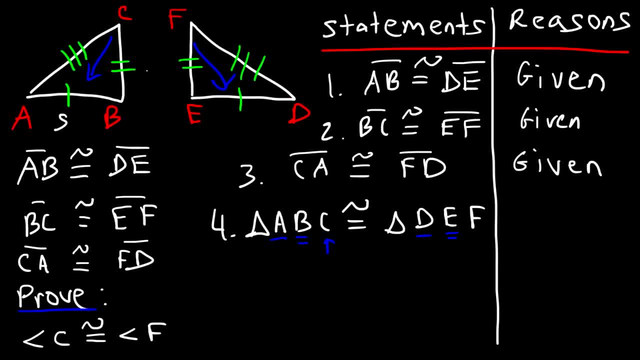 say that these two triangles are congruent based on the side side side postulate. Now we've used statements 1,, 2, and 3 to show that those three sides are congruent, So let's put 1,, 2, and 3.. 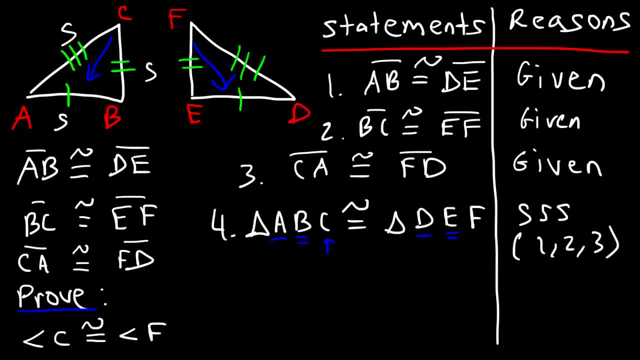 Now, once you prove that the two triangles are congruent, the last step in my experience, is always going to be CPCTC. Now you can prove that any corresponding parts of these two triangles are congruent. In this case, 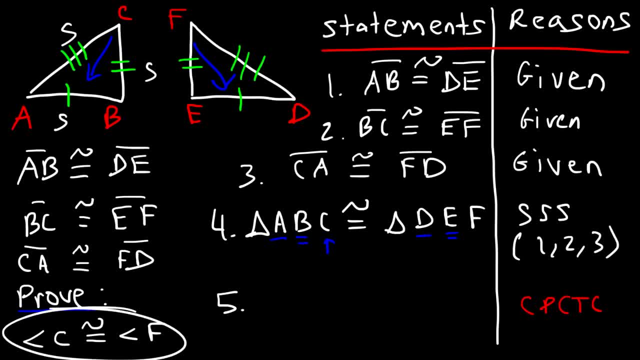 we can say the final sentence or make the final statement So we can say that angle C is congruent to angle F. based on CPCTC, Corresponding parts of congruent triangles are congruent And that's it for this problem. 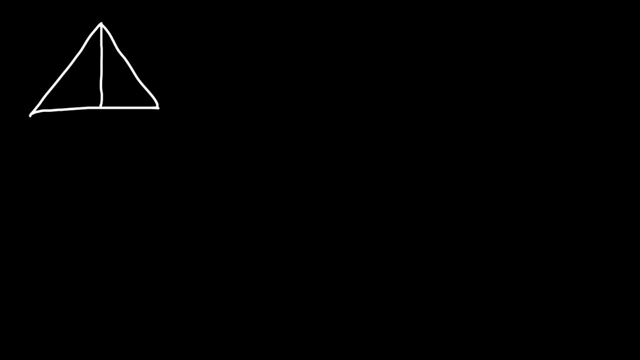 Now let's work on another example. So let's say this is A, B, C and D, And you're given that BD is perpendicular to AC And also B is the midpoint of AC. So your task is to: 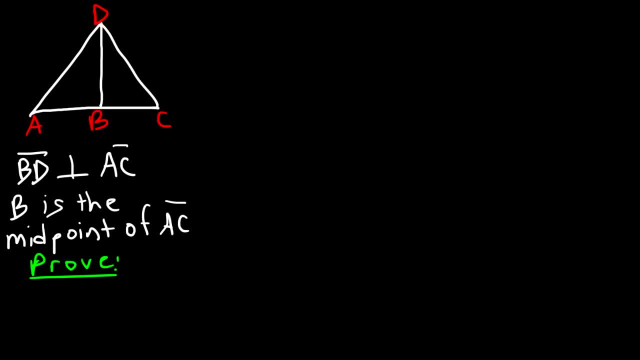 prove that AD is congruent to CD. So feel free to pause the video. if you want to try this problem, So prove it using the two column proof. So let's start with number one. So we're given that BD. 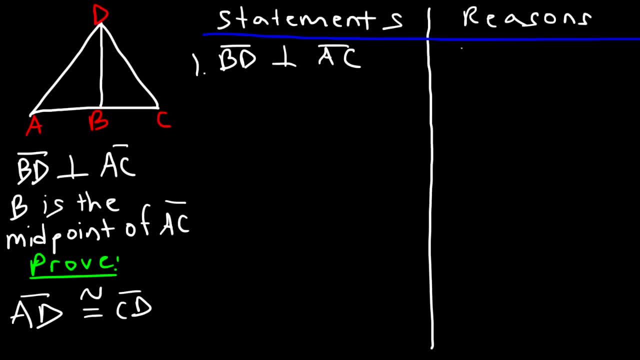 is perpendicular to AC, And let's write given. So what conclusions can we draw from that statement? If BD is perpendicular to AC, what do we know? Perpendicular lines form right angles, So that means that ABD is the right angle. 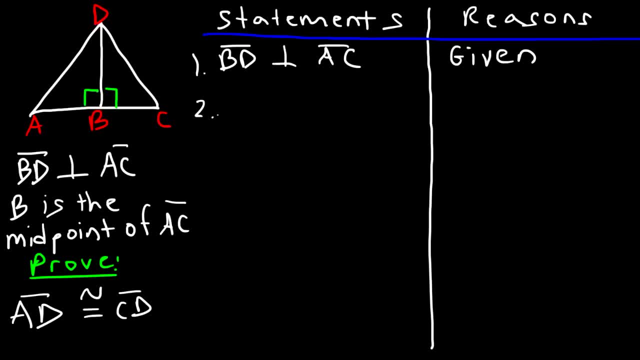 and DBC is the right angle. So we can make another statement. We can say that angle ABD is congruent to angle CBD, And the reason for that? perpendicular lines form right angles. Now what else can we say? Well, we have another. 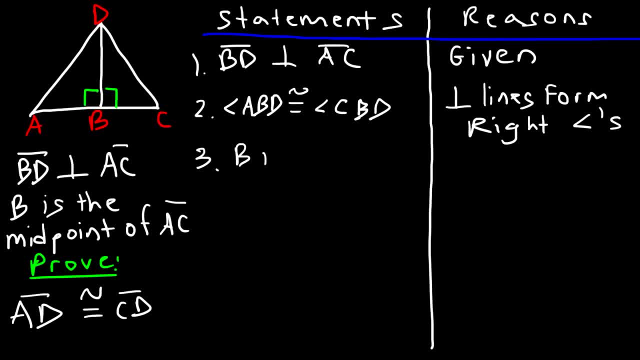 given statement, and that is that B is the midpoint of segment AC, And so that's given. Now, what conclusions can we draw from that given statement? If B is the midpoint of AC, what do we know? Well, if B is the midpoint, 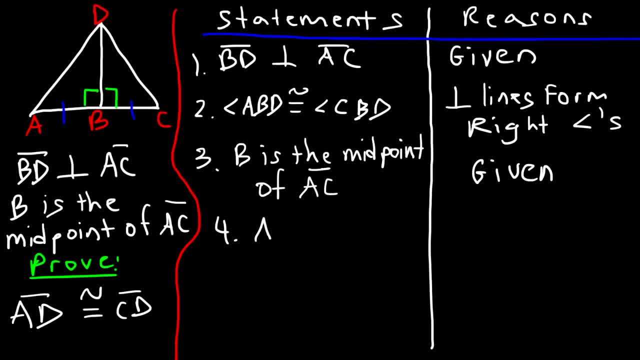 that means AB is congruent to BC. They have to be of the same length, And the reason for that is definition of a midpoint. Now what else can we say? What else do we need to prove that the two triangles are congruent? 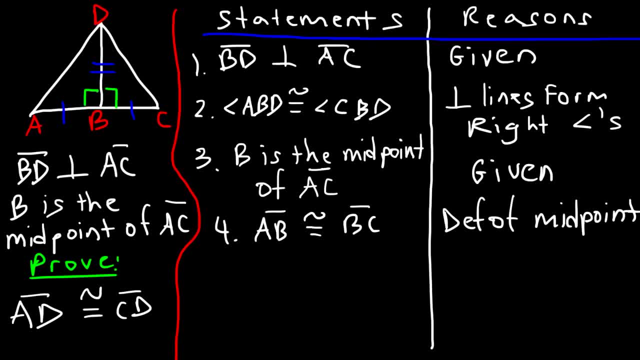 Now notice that triangles ABD and CBD share a common side, And that side is BD. So we can say that BD is congruent to itself According to the reflexive property. Now we can prove that the two triangles are congruent. 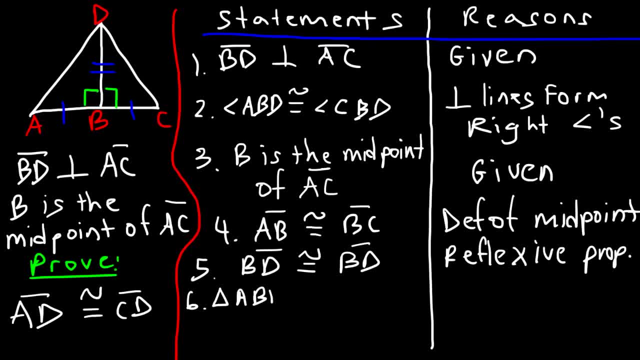 So we can say that triangle ABD is congruent to triangle CBD, And the reason for that? we have a side, an angle and a side, So it's the side-angle-side postulate, And to prove it we've used statements. 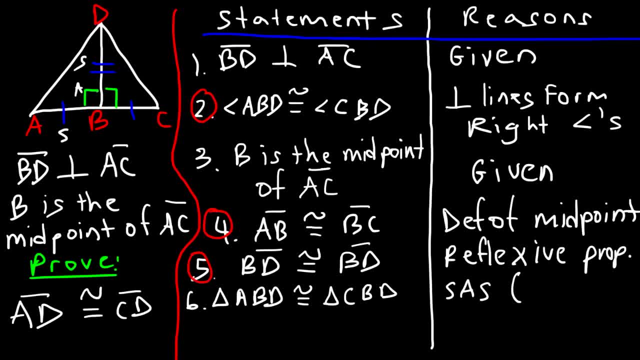 2,, 4, and 5.. Now, once you prove that the two triangles are congruent, the last step is going to have this statement, The statement that you're trying to prove That AD is congruent to CD, And all you've got to say is CPCTC. 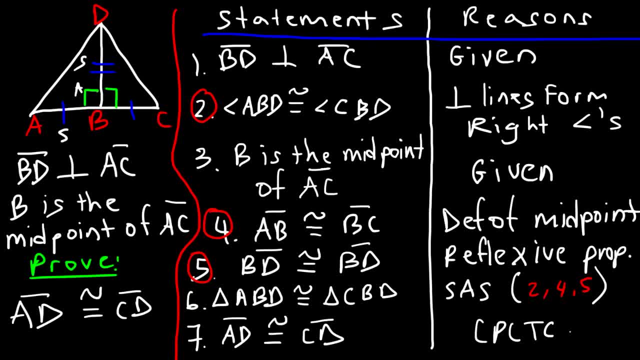 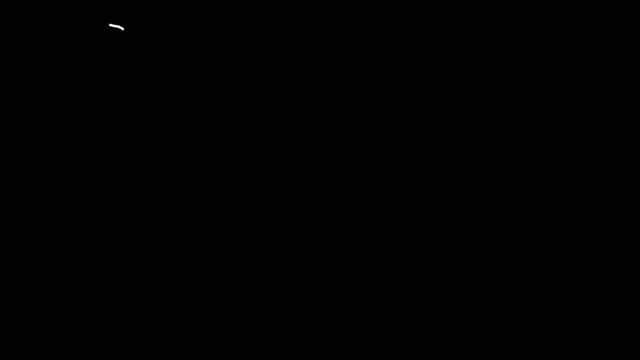 That's the reason: Corresponding parts of congruent triangles are congruent, And then this problem is done. That's it. Let's work on another example. Let's say: this is the center, And let's call this point A, B. 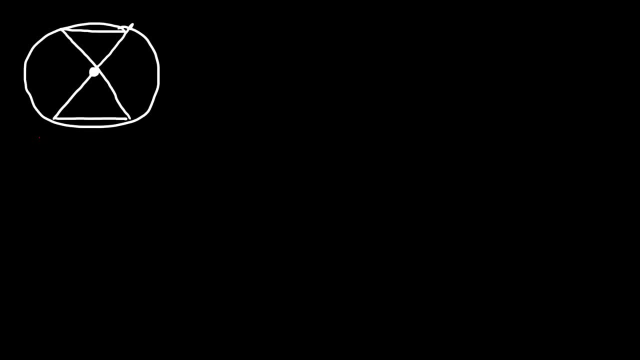 C and D, And so you're given that E is the center of the circle And you're, that's all you're given. Just E is the center of the circle. So you're given that And you want to prove. 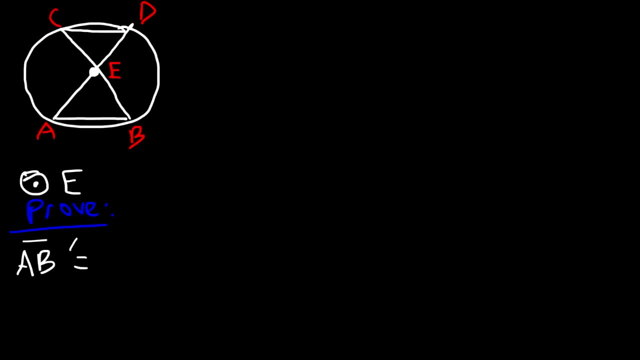 that segment AB is congruent to segment CD. So all you know is that E is the center of the circle. Prove that this segment is congruent to that segment. Alright, so let's begin. Let's start with our two-column proof. 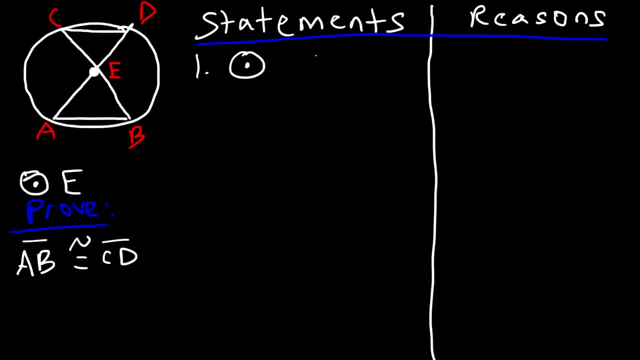 So number one point: E is the center of the circle, And so that's given to us. Now, what conclusions can we come up with, knowing that E is the center of the circle? Now, you need to know that the distance between 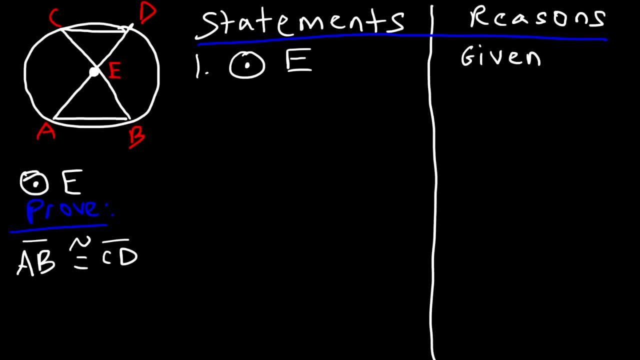 the center and any point on the circle is the radius of the circle And the radius of the circle is the same anywhere on the circle. So that means that AE is the radius of the circle, EB is the radius, as well ED and CB. 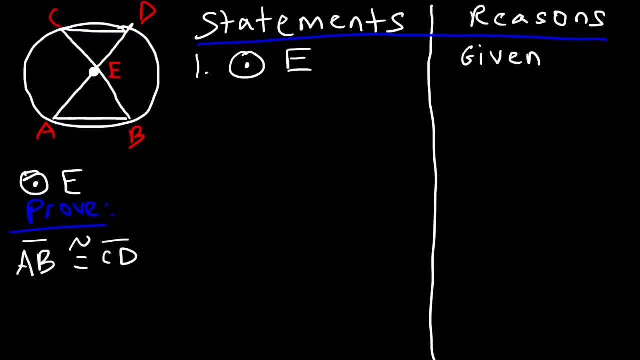 are all radii of the circle, Which means they're all congruent to each other. But because we wanted to prove that the two triangles are congruent, let's take this one step at a time. So for statement two, we're going to say that AE. 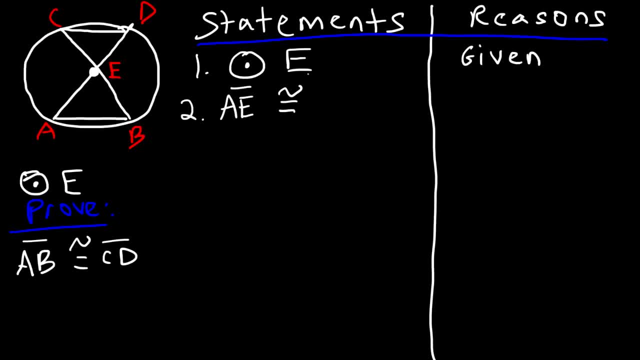 is congruent to DE. So here's AE that's congruent to DE. Now we can also say that BE is congruent to CE, Because they represent the radius of the circle as well. But I'm going to use a different tick mark. 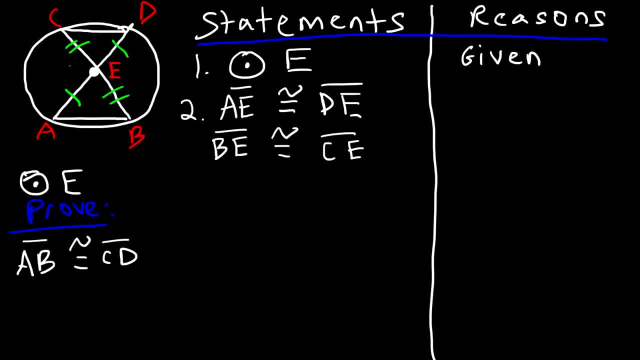 So we can see that we have two sides of the two triangles that are already congruent. Our goal is to prove that this triangle is congruent to that triangle. If we can do so, then using CPCTC, we can say that: 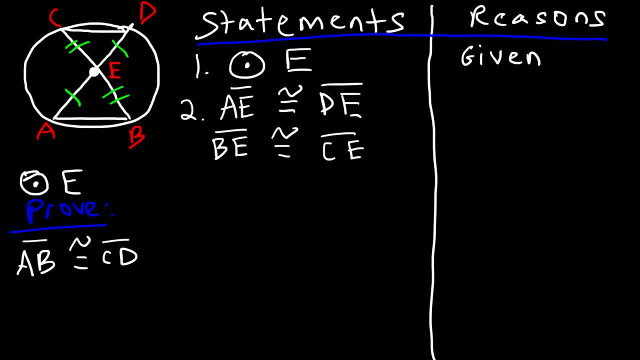 this statement is a true statement. So what should we put in the second column for this statement? What's the reason? Well, the reason is simple: All radii of a circle are congruent. So that's the reason. Now let's move on to step three. 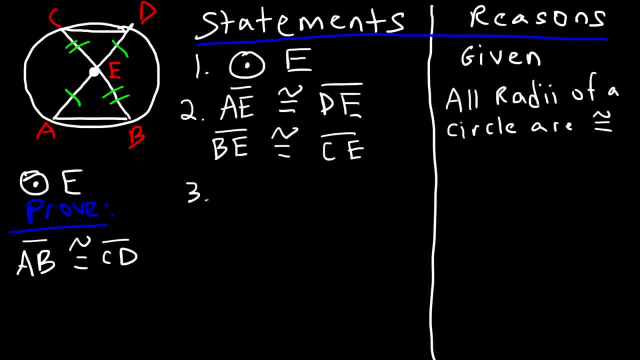 What else can we say? Whenever you have two lines or two segments that intersect each other- well, technically two lines- they will always produce vertical angles And vertical angles are congruent. So what we can say is that angle A, E, B. 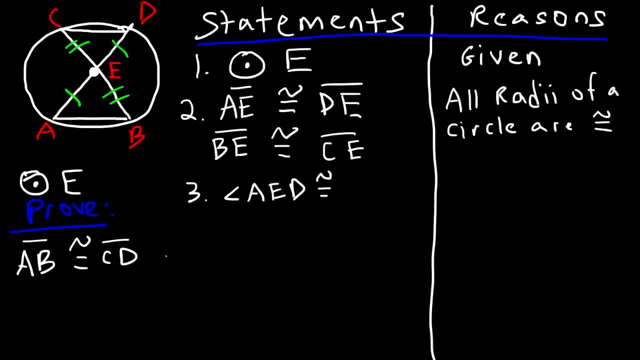 is congruent to which angle. So this is A E, B And we know that it's congruent to this angle, But how should we call it? Should we say it's angle D, E, C or C E D? Think about it. 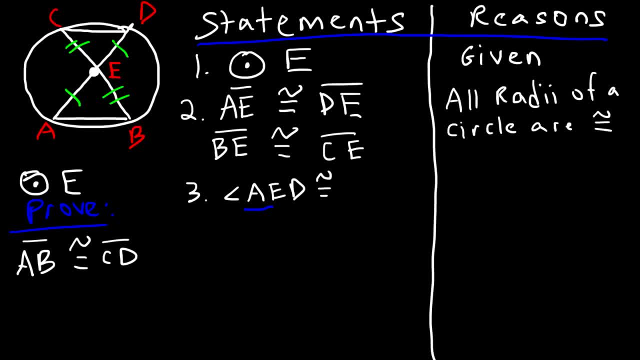 Well, let's find out. So A matches to what letter? Does A match C, D or E? So notice that A is opposite to the side with two marks. So therefore D is opposite to that same side, But technically it turns out that 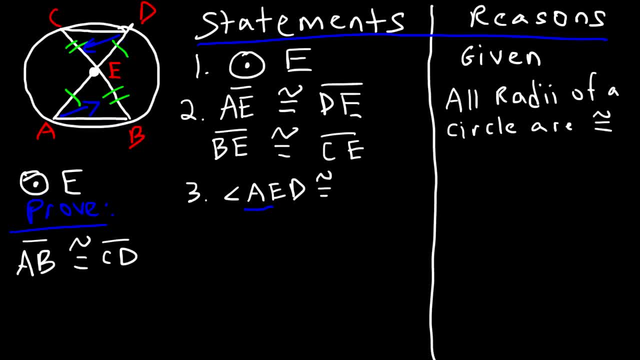 both answers could work Because, since every side represents the radius, all four angles must be equal to each other. But if they were different, I would say that A and D would match up because they point to the same side with the same number of tick marks. But for this. 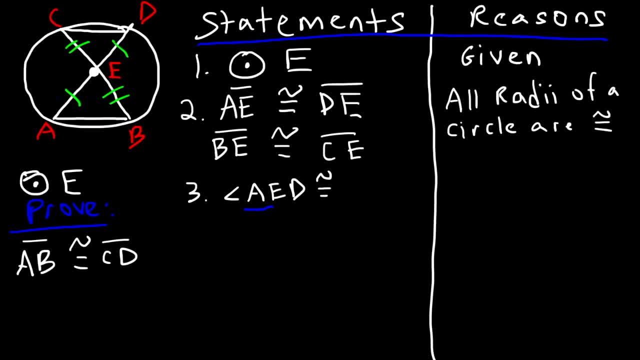 particular problem. everything's the same. These two sides are equal, So therefore these two angles are congruent. So you could say D E C or C E D for this particular example, But for other examples I would keep it safe and say that A matches. 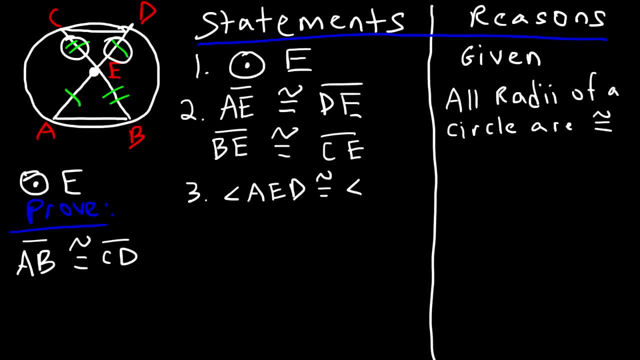 with D if these two are different. So this is going to be equal to angle D E C. Now why can we say that? So, as we mentioned before, the reason why they're congruent is because they're vertical angles. 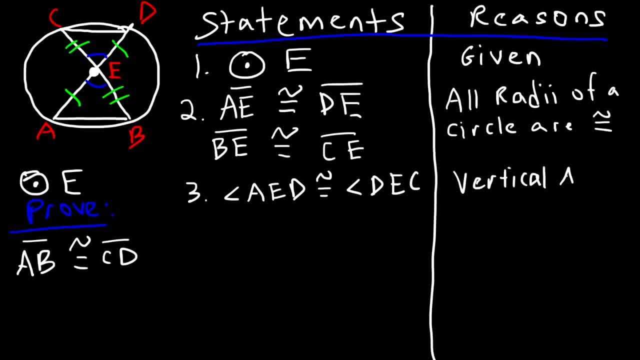 So the reason is: vertical angles are congruent. Now number four. So now we can say that the two triangles are congruent, So triangle A, E, B. Oh, this is supposed to be a B, by the way. I don't know why I made that a D. 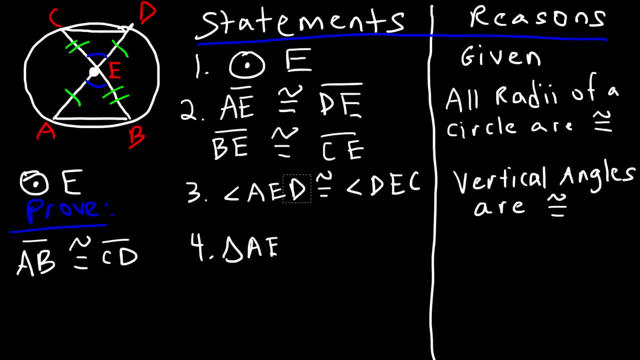 So let's fix that. So that was supposed to be angle A B E. excuse me, A E B. It's congruent to D E C. So now triangle A E B is congruent to triangle D E C. I'm making too many mistakes here. 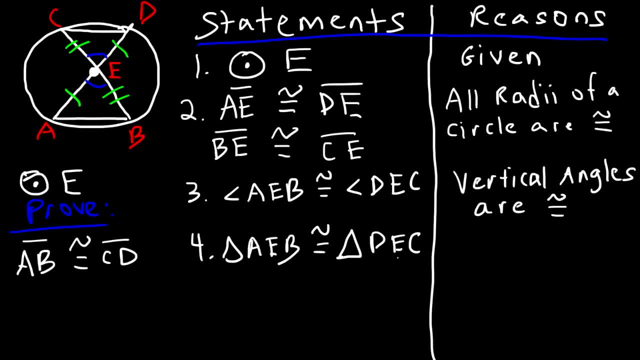 Now, what's the reason? What postulate can we use that to prove these two triangles? So we have a side and angle and a side, So it's S A S. Now what statements did we use to prove that those two triangles are congruent? 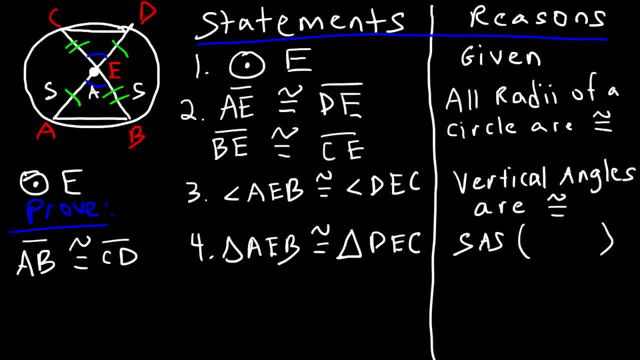 So for this side, we use statement two, which states that A? E is congruent to D E. So we gotta go in order. Next we have the angle. So we use statement three to prove that the vertical angles are congruent. 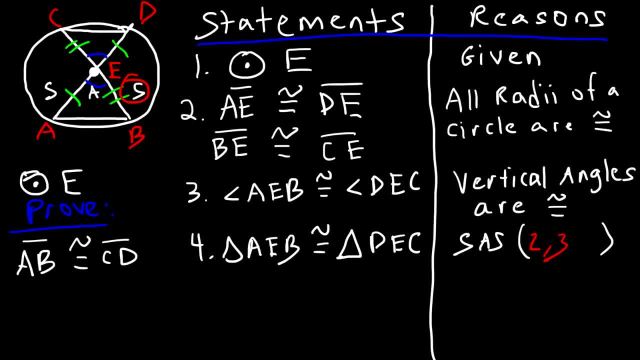 And then this side is based on statement two, Where B E is congruent to C E, So it's gonna be two, three and then two. So now that step four is finished and that the two triangles have proven to be true, 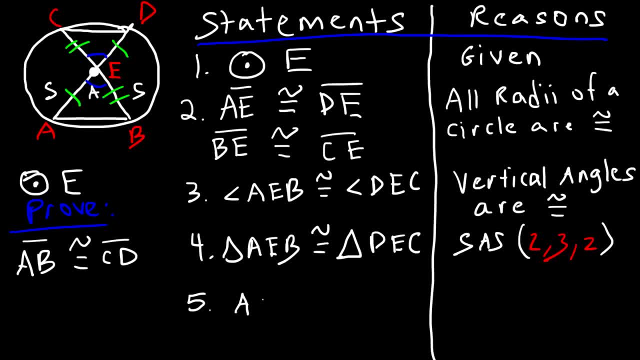 we can now move on to our last statement, which is the statement that we're trying to prove, And that is that A, B is congruent to C, D, And the reason is: C, P, C, T, C- Corresponding parts of congruent triangles are congruent. 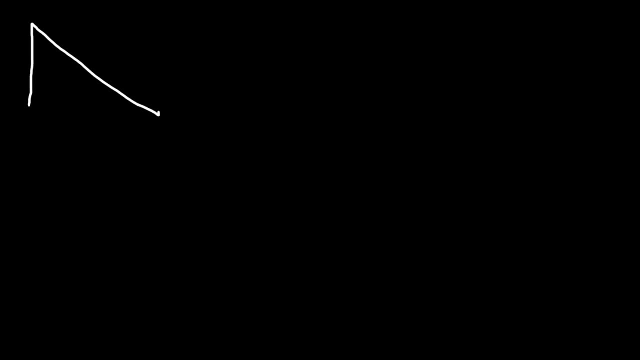 Now let's work on another example. So let's call this A, B, C, D, E. Now we're given that A, B is parallel to D, E, And we're also given that segment B, D bisects segment A, E. 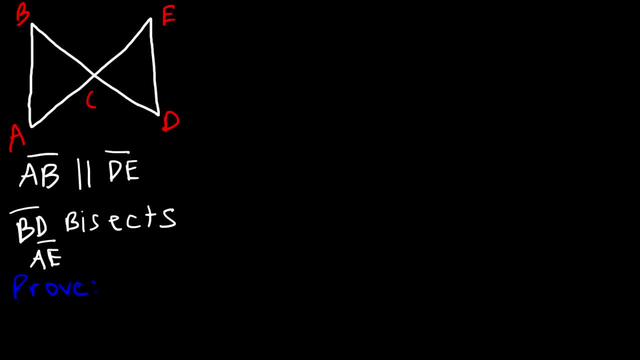 So, with this information, prove that segment A B is congruent to segment D E. Now, at this point, if you want to try the problems, just pause the video and work on it and see if you can get the right answer. 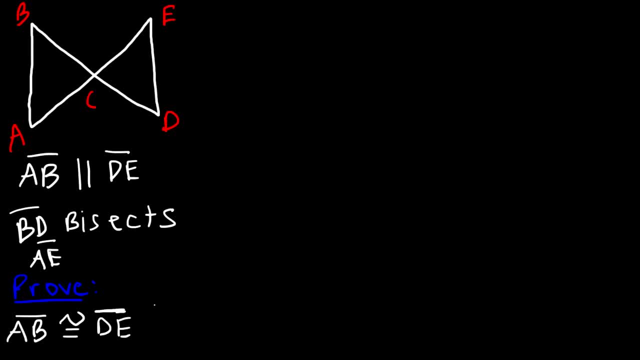 The best way to learn is by practicing these problems and then, as you begin to do them, the more that you do these problems, the more you understand what to do next, what reasons to put and just how to go about to solve these types of things. 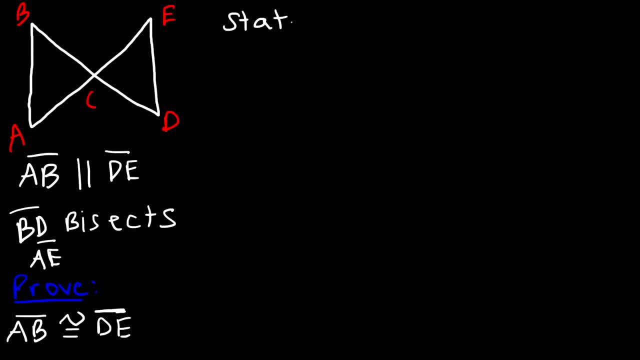 So let's begin. So in the first column let's put statements And in the second one reasons. So let's write the given: A, B is parallel to D, E, So that's a given, And let's mark it on a graph. 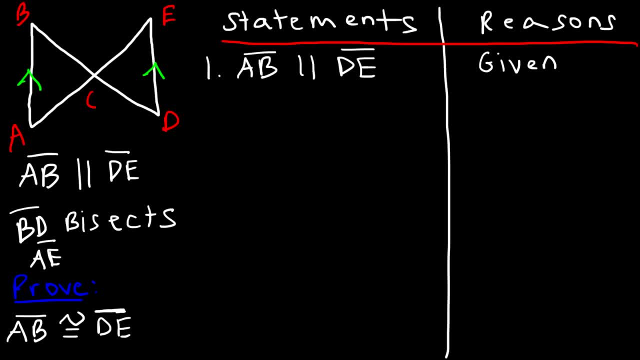 So this is the symbol to indicate that two lines or two segments are parallel. Now, what can we figure out with this information? So, knowing that A, B is parallel to D, E, what can we deduce Whenever you have parallel lines? 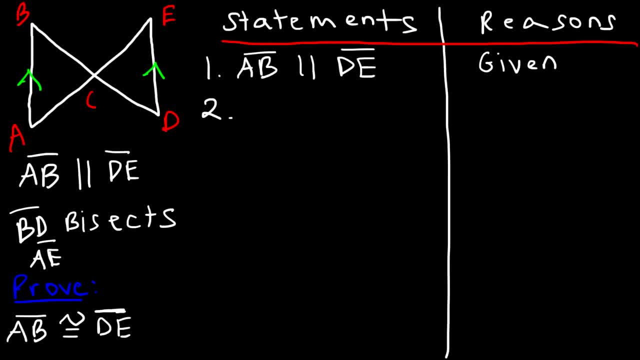 look for alternate interior angles. So we could say that angle A is congruent to angle E. You could also say that angle B is congruent to angle D, But we'll take it one step at a time. So let's say: 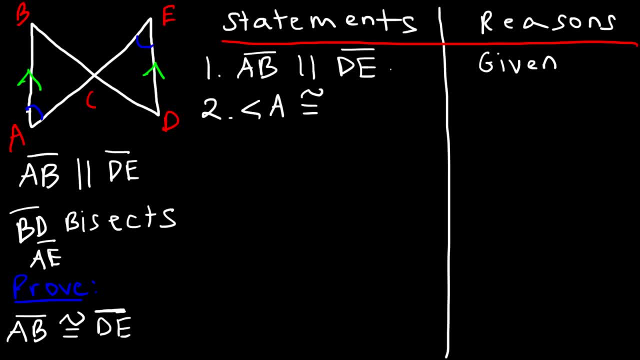 that angle A is congruent to angle E. Now what reason can we put? So? here is what we need to say: Alternate interior angles are congruent. So that's the reason. Now, next let's write that B, D, 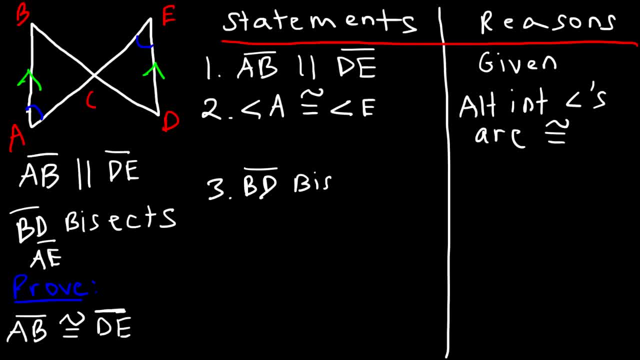 bisects segment A- E. So this is B- D and it splits A- E into two equal parts. That means that A- C is equal to C- E, And for statement three that's simply a given. But for statement four we could say that A. 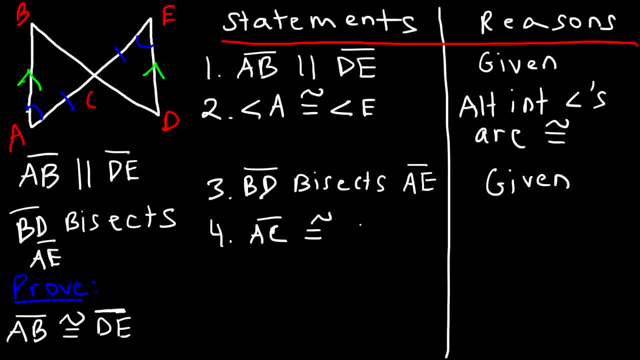 C is congruent to C- E. And a reason: definition of a segment bisector. Now number five. We could say that these two angles are congruent because they represent vertical angles. So we're going to say that angle A, C, B. 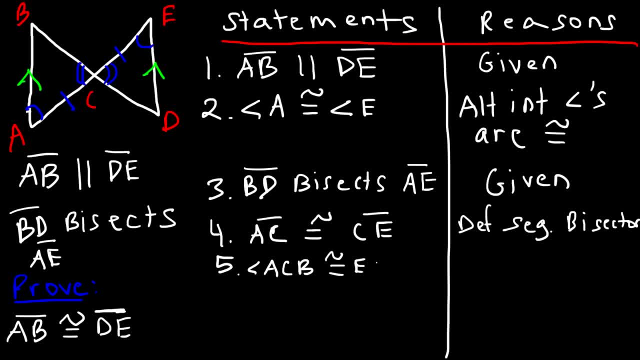 is congruent to angle E, C, D. So notice that D corresponds to B. They're opposite to two congruent sides, So I have to make sure that B matches with D. And a reason: Vertical angles are congruent. Now let's move on to 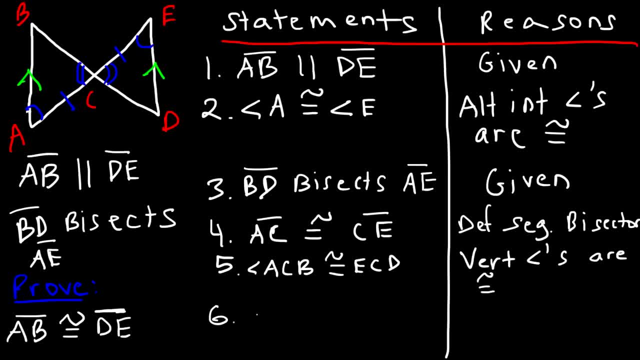 statement six. So we can now prove that the two triangles are congruent by the angle side angle postulate. So triangle A C B is congruent to triangle E C D, And so the reason for that is the side angle side postulate. 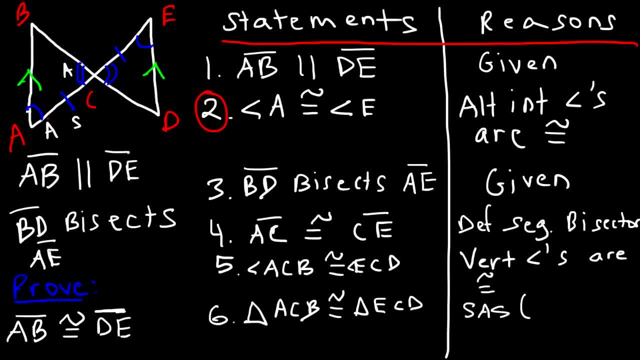 And first we had angle two which corresponds to- I mean statement two, which corresponds to that angle. Angle A equals angle E. Next we prove that the sides were congruent. So A C is equal to C E. So that's statement four. 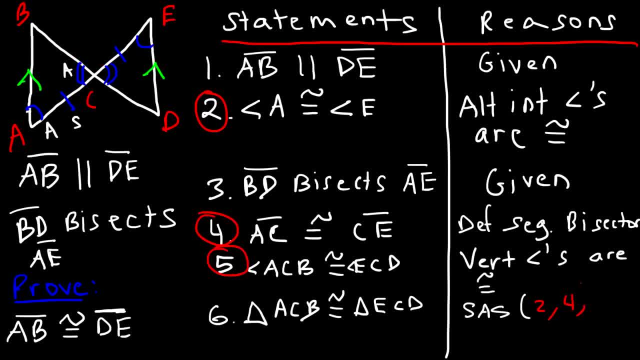 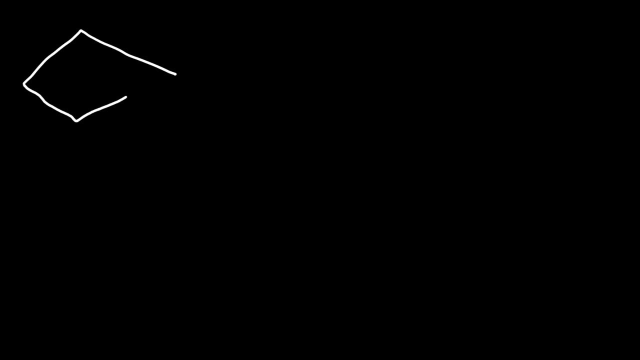 And then the vertical angles are congruent, which was based on statement five. So now we can make the final statement that segment A B is congruent to segment D, E using C, P, C, T, C. So let's call this A B. 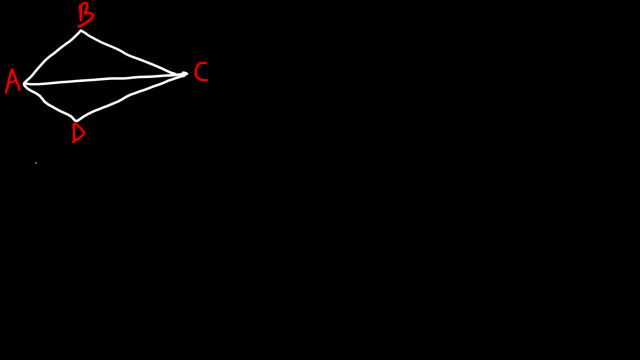 C and D. So in this problem we're given that angle B is congruent to angle D And also that ray A C bisects angle B A C. Actually not B A C, but rather B A D. So 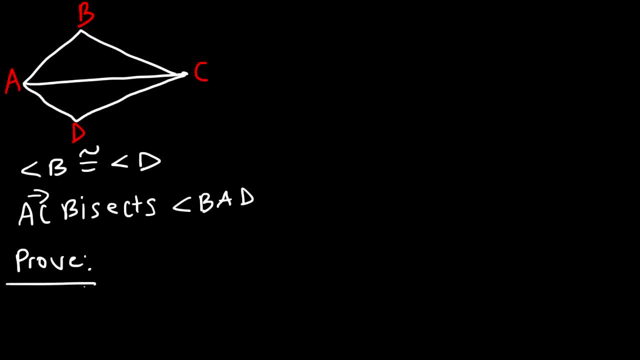 go ahead and prove that segment B C is congruent to D C, So feel free to try this problem. Okay, let's start with number one. So we're given that angle B is congruent to angle D, So that's a given. 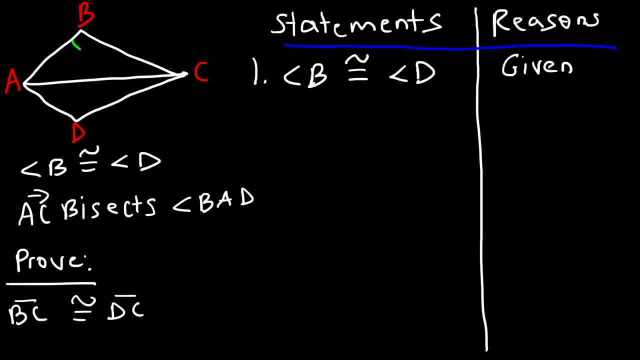 And now let's mark it on the graph. So B is equal to D. Now what else can we do? So number two: we know that ray A C bisects, bisects angle B A D. So this is ray. 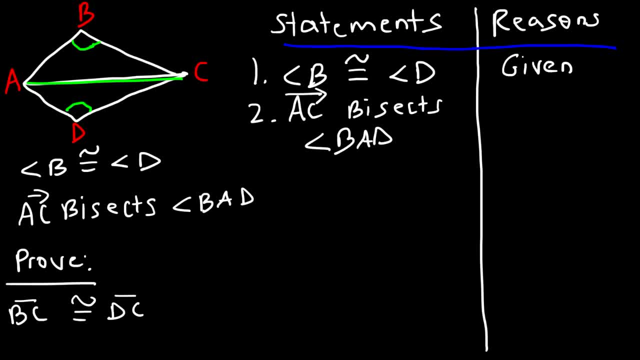 A C. It emanates away from point A, And so it bisects angle B A D into two congruent angles, which means angle B A C is congruent to angle D A C. So number two, this is a given. 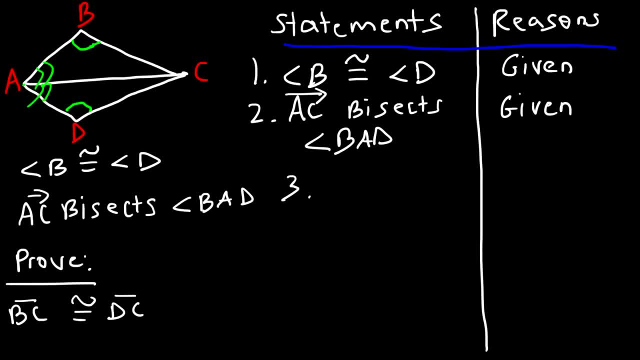 But in number three we can say that let's put a line to separate these two, The given, from the actual problem. So in step three we can say that angle B A C is congruent to angle D A C And the. 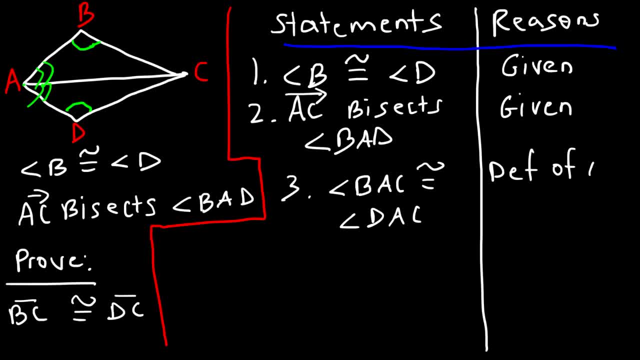 reason for that is definition of an angle bisector. Now let's move on to our next step. In step four, we can say that A- C is congruent to itself due to the common side that we see here, And that's based. 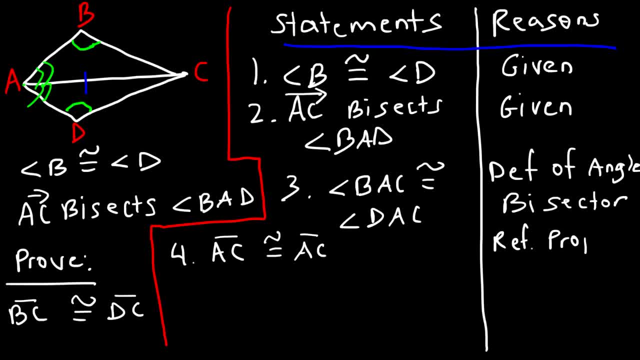 on the reflexive property. Now step five. we can show that the two triangles are congruent using the angle angle side theorem. So we can say that triangle B A C is congruent to triangle D A C, And this is based on the angle. 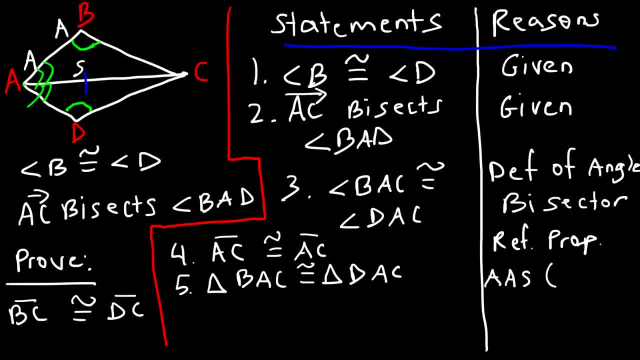 angle side postulate. So the first thing we did, we proved that B is congruent to D. So that was the first angle we proved and that was based on statement one. And then we showed that angle B A C and D A C are congruent. 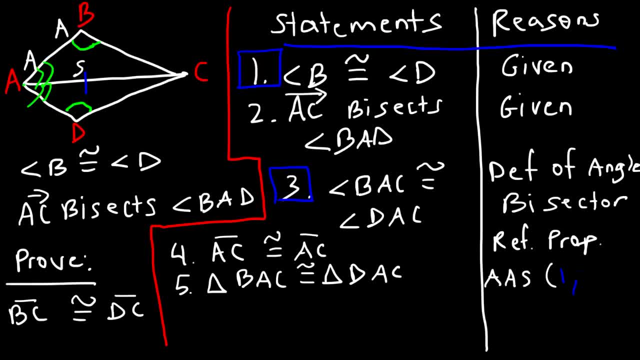 So that's based on statement three. And finally, the common side, which was the S symbol, and that's for statement four. So it's based on statements one, three and four. And now let's make the final statement that 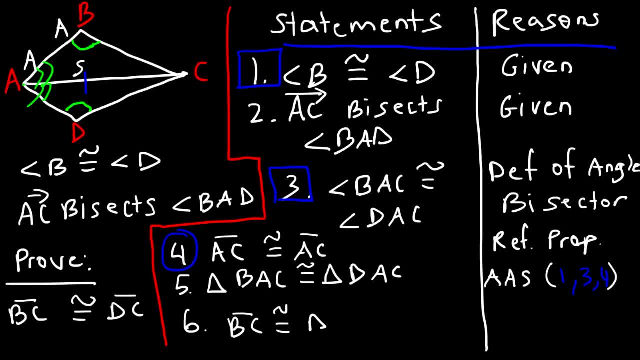 segment B C is congruent to D C. So here is B C and this is D C, So they're the same. And the reason for that: as always, C, P, C, T, C- Corresponding parts of congruent triangles are congruent. 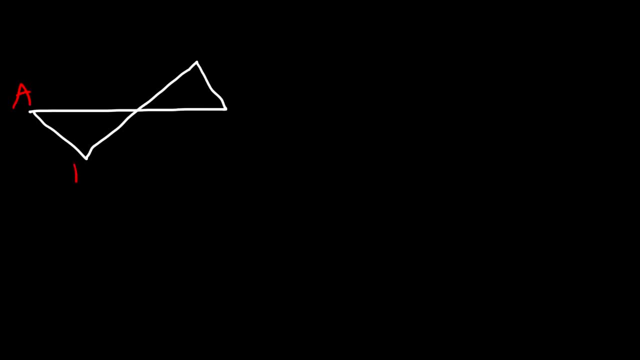 So let's call this A, B, C, D and E. So we're given that angle one is congruent to angle two. You might be wondering: where is angle one? So this is going to be angle one and here is angle two. 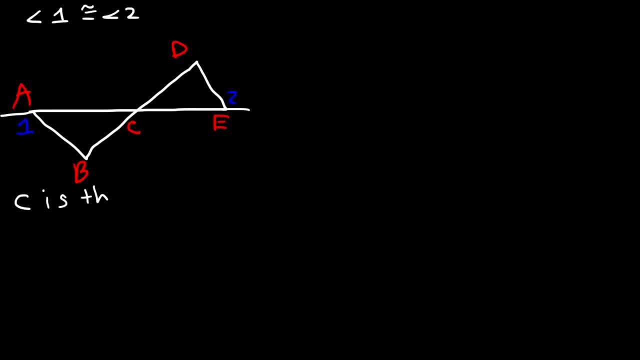 And also C is the midpoint of, of, of A E, of A E. So go ahead and prove. So go ahead and prove that segment A, B is congruent to segment E, D to segment E D. 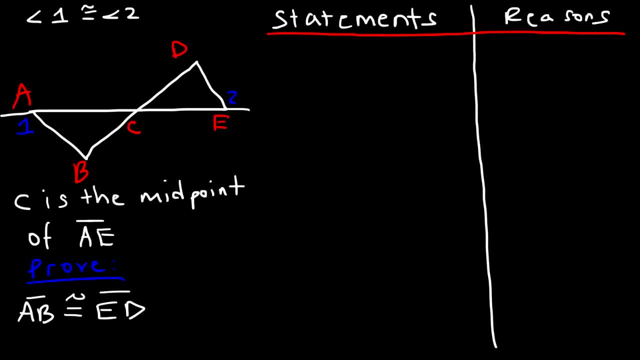 So number one let's start with. let's see the angle. So angle one is congruent to angle two, So that's given. So our goal is to prove that triangle A, B, C is congruent to. 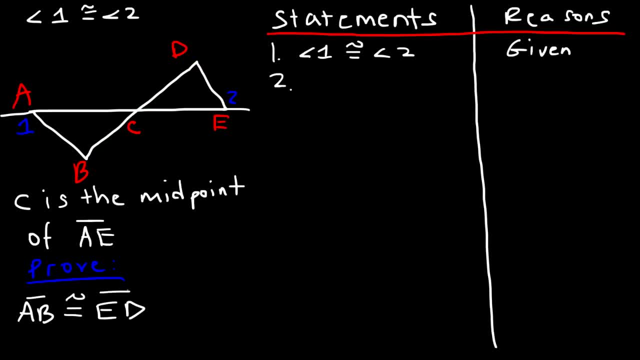 E, D, C. If we can do that using C, P, C, T, C, we can prove that this statement is correct. But angle one and two are outside of those two triangles And we need angles that are inside the two triangles, So let's call this angle three. 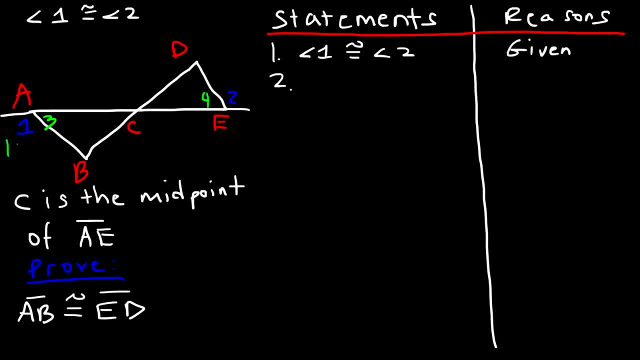 and angle four. Now if angle one is 100 degrees, that means angle two is 100.. Now one and three forms a linear pair. They're supplementary. That means three has to be 80 and four has to be 80.. 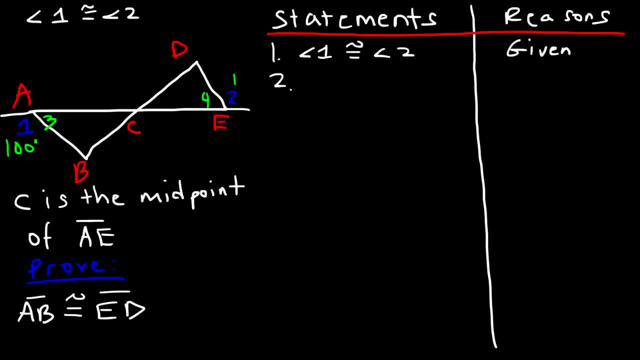 So therefore, angle three and angle four are congruent to each other. So let's write that in the next statement: Angle three is congruent to angle four And the reason for that is: supplements of congruent angles are congruent to each other. 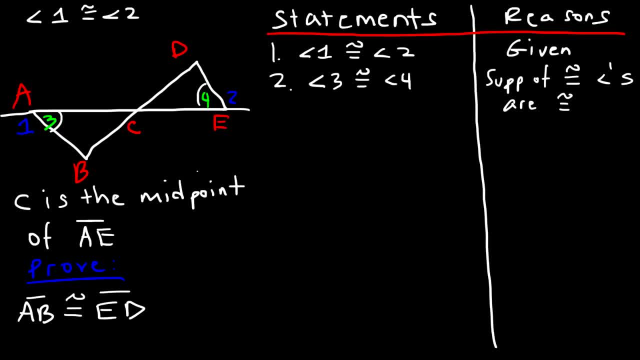 And so let's mark that. So three is congruent to four. Now let's move on to the next part. C is the midpoint of A, E, And that's a given. So what can we conclude? any time we have a midpoint, 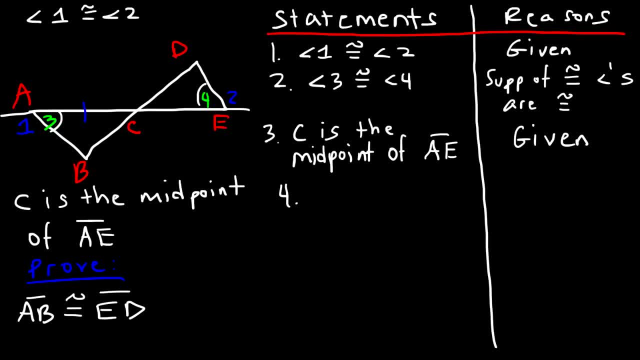 A midpoint separates a segment into two equal segments. So we could say that segment AC is congruent to segment CE And the reason is definition of a midpoint. Now the last thing we could do is prove that these angles are congruent. 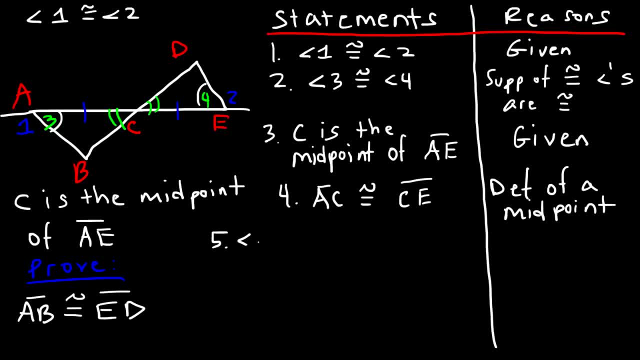 So in step five we could say that angle ACB is congruent to angle ECD. And the reason: vertical angles are congruent. Now let's move on to step six. So now we could prove that the triangles are congruent. 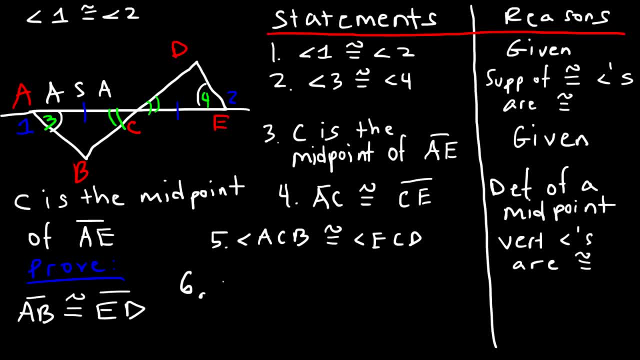 We have an angle, a side and an angle. So let's say that triangle ACB is congruent to triangle E CD And that's using the side angle. actually, that's the wrong one. It's the ASA angle, side angle. 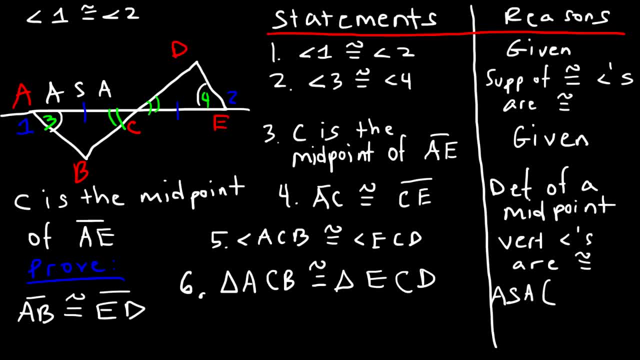 postulate, And the first angle that we proved was angle three is congruent to angle four, So that's based on statement two. And then for the S, we prove that AC is congruent to CE, So that's statement four. 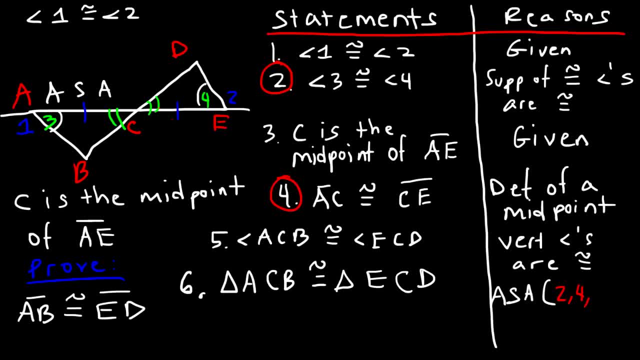 And then statement five: the vertical angles are congruent, So it's based on two, four and five angle, side angle. And now, finally, we could say that segment AB is congruent to segment ED, based on CPCTC. 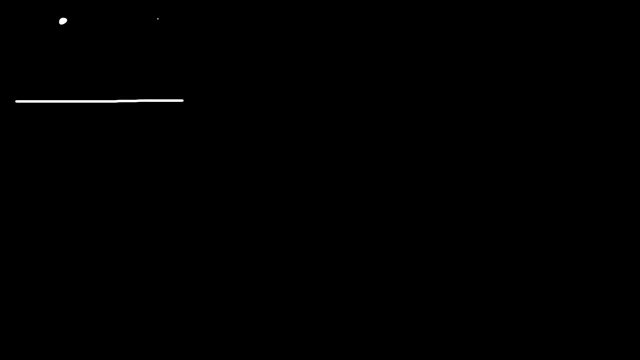 Now let's try another problem, So this one might be a little bit harder than the other ones that we've been dealing with so far. So let's call this A, B, C, and then this is going to be D and E. 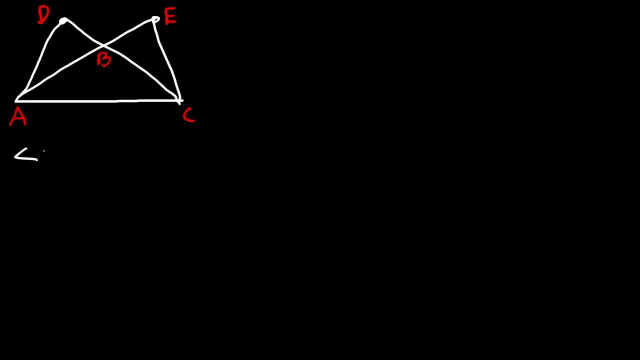 In this problem. we're given that angle one is congruent to angle two. So this is angle one and here is angle two. And we're also given that DC is congruent to EA. Our task is to prove that. segment AD. 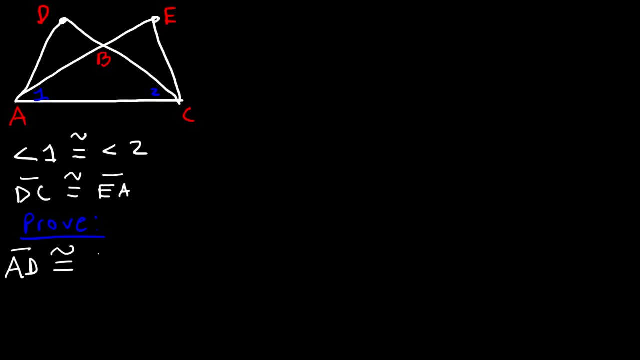 is congruent to segment EC, So go ahead and work on this problem. So, number one: let's start with the angles. Angle one is congruent to angle two, And that's given. Now notice that angle one and two are part of. 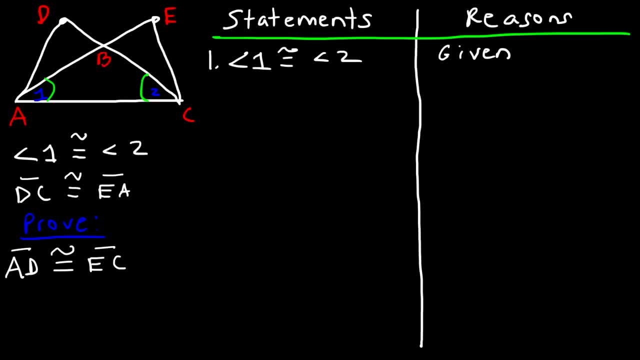 a single triangle as opposed to two separate triangles. So what can we conclude from this information And also what is our goal? In order to prove that AD is congruent to EC, we need to prove that triangle ADB and this triangle. 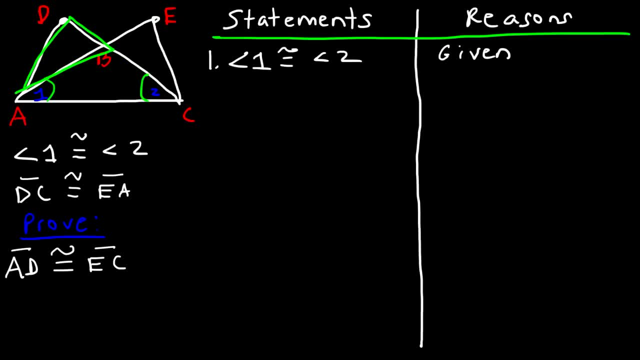 CEB, they have to be congruent. Or if you can prove that the triangle ADC is congruent to AEC, you can also prove that AD is equal to EC. Depending on which one is easier, I'm going to go with. 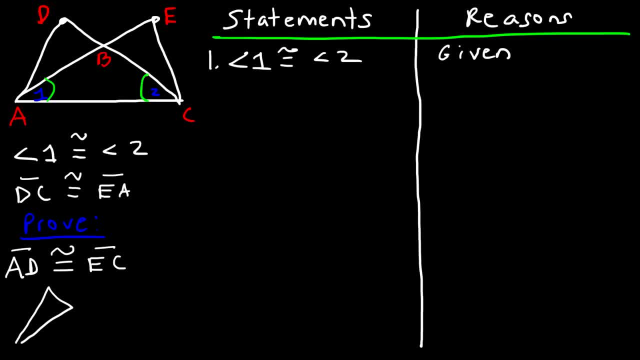 the first two triangles that I drew, So let me redraw. So this is ABD and here we have CBE. So if we can prove that those two triangles are congruent, then we can easily prove that AD is congruent. 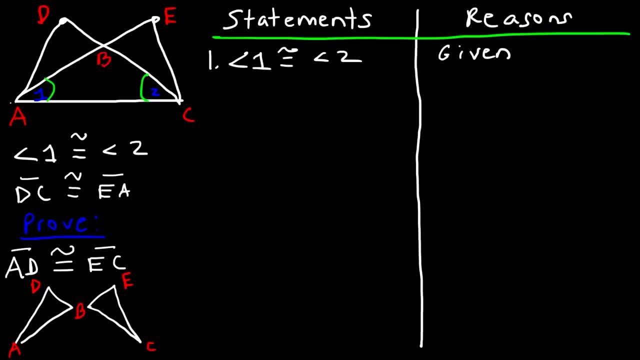 to EC. Now let's focus on triangle ABC. That triangle is an isosceles triangle because two angles are the same, which means that the sides across those two angles, AB and BC, must be equivalent, So AB is congruent. 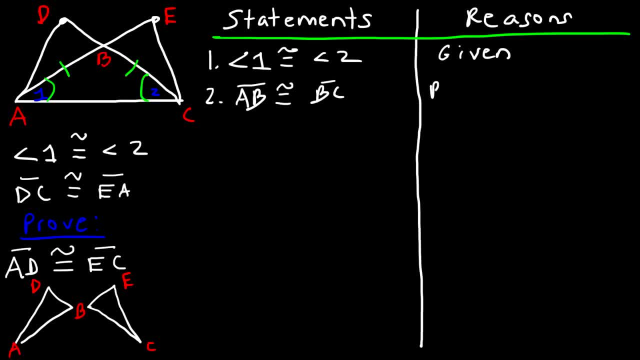 to BC And we could say the reason for that is the base angle theorem Within a single triangle. if the angles are congruent inside a single triangle, then the opposite sides are congruent. So far we've been dealing with congruent angles of two separate 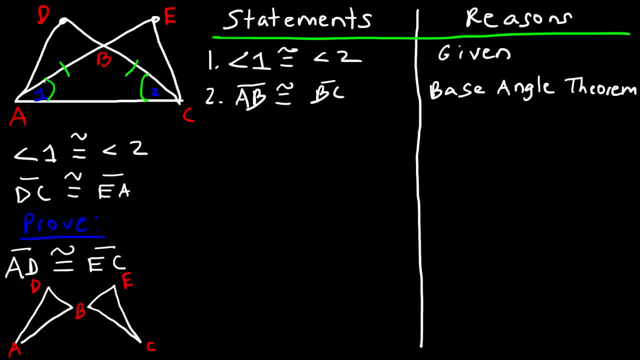 triangles, but whenever you have within a single triangle, if two angles are congruent, then the opposite sides will be congruent, based on the base angle theorem. So right now we know that AB is congruent to BC. Now what else do we know? 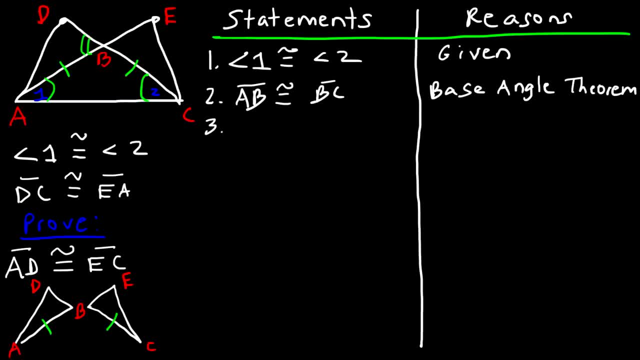 So notice that angle DBA and EBC, those are congruent angles. They're vertical angles And we know that vertical angles are congruent, So let's mark that. So these angles are congruent. And now we just need one more detail, one more. 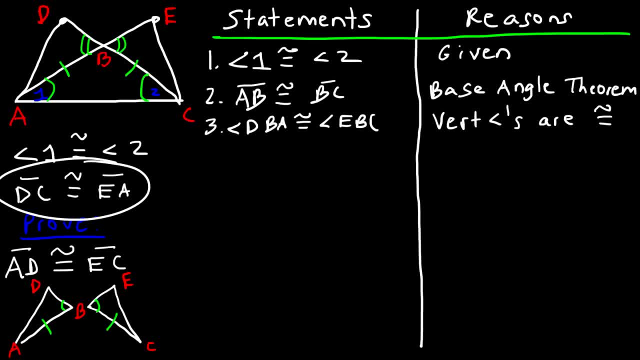 piece of information. So let's use the fact that DC is congruent to EA And that's given. So here is DC and here is EA, So they're congruent, and we know that BA is congruent to BC. 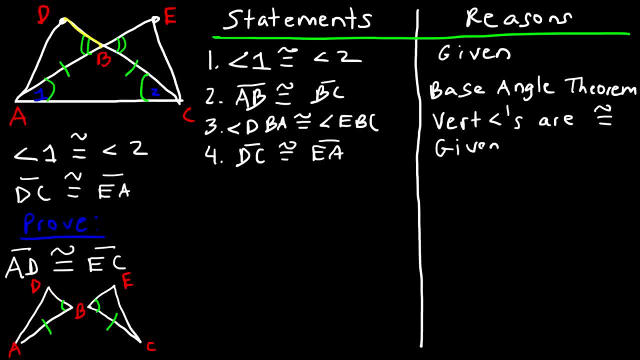 Therefore, by intuition, you can see that DB is congruent to BE. We just have to show it. Once we can prove that DB is equal to BE, we can prove that these two triangles are the same. So we need to perform. 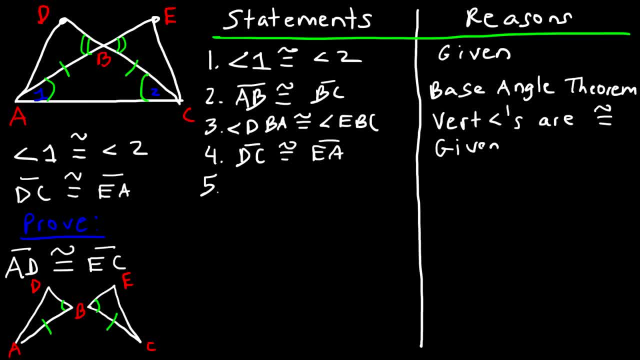 segment addition. So whenever you need to perform some sort of mathematical operation with segments, you need to change this into a certain value. So we're going to say that DC is equal to EA. This is definition of congruent segments. Now notice that DC 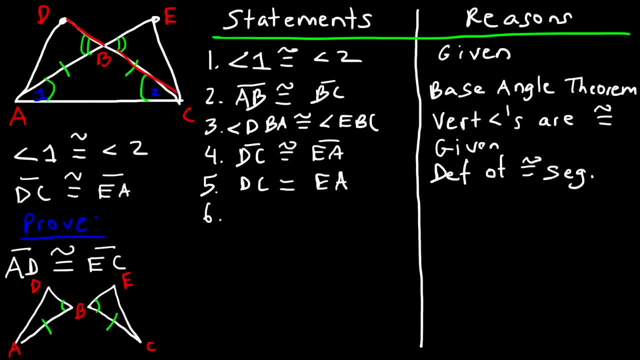 is basically DB plus BC. If you add those two, you're going to get DC And in addition to that, EA is basically AB plus BE. That will add up to segment EA. So let's replace DC with DB plus BC. 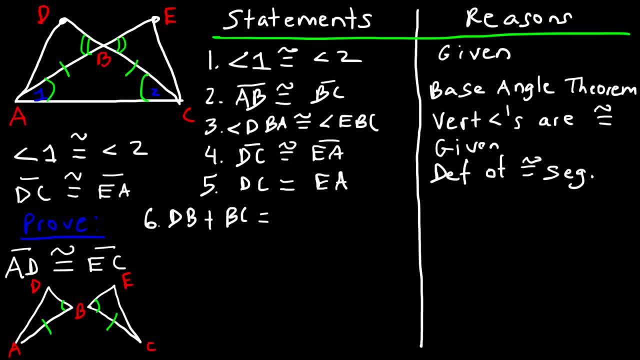 And then let's replace EA with AB plus BE, And so whenever you're breaking down two segments or a large segment into two segments, or if you want to add two small segments into a larger segment, the reason or the property. 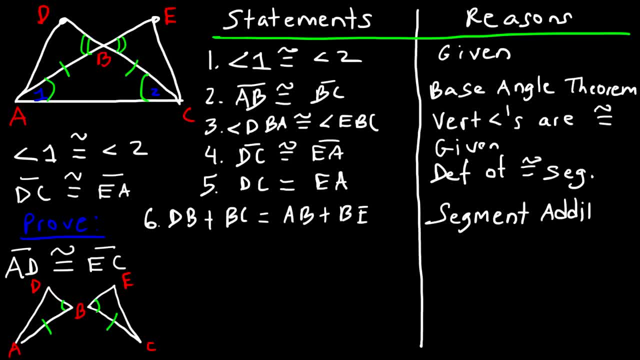 is segment addition. Now, what do you think we should do at this point? What's our next step Now? looking at statement two, notice that AB and BC are congruent. So we could therefore replace BC with AB. So in step seven, 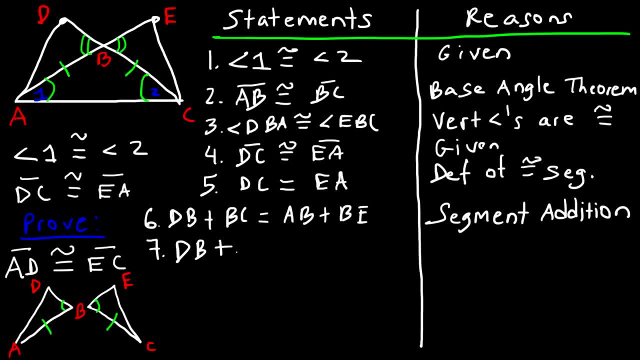 we're going to have DB plus AB is congruent to AB plus BE. So we've replaced or substituted BC with AB. So this is going to be the substitution property. So I'm just going to write substitution, but on the test I would put the word property as well. 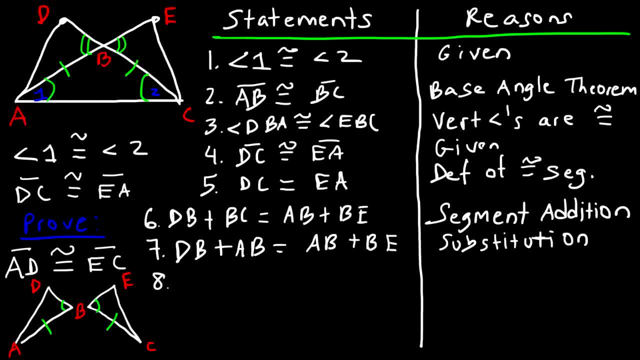 I'm running out of space Now in step eight, because we have AB on both sides. we can subtract both sides by AB. Thus it's going to cancel these two, And so we're going to be left with: DB is equal to AB. 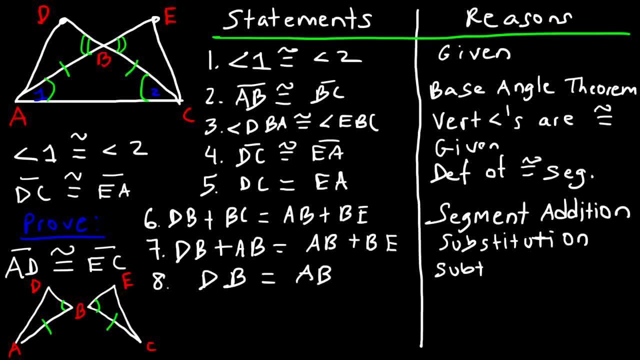 according to the subtraction property. Now, in step nine, we could say that segment DB is congruent to segment AB. And why can we say that? Definition of congruent segments? So now that we have that again, we could say that we could put the marks: 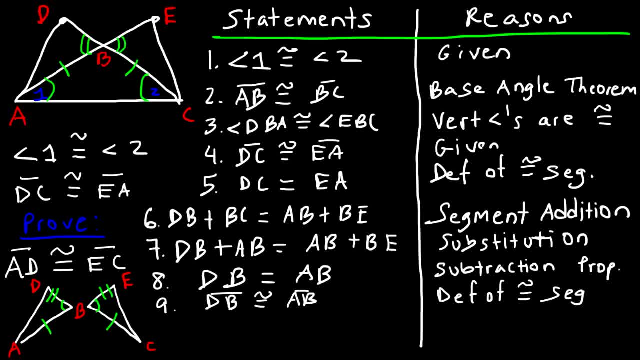 on the graph DB is congruent. I don't know why I put AB. Let me fix that. AB should be cancelled. That should not be an AB. That should be gone. So it should be BE For long problems, it's easy. 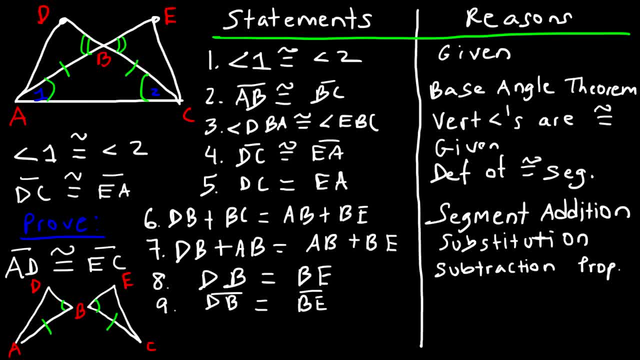 to make a mistake. So DB is congruent to segment BE, And let's rewrite this Definition of congruent segments. Let's put the mark here: DB is the same as BE, So now we could show that these triangles are congruent. 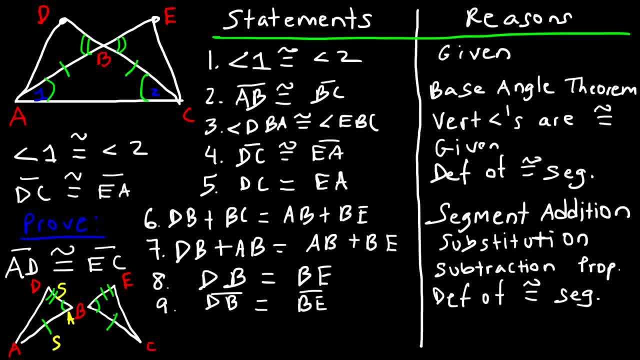 based on the side angle side postulate. So for statement ten we're going to say that triangle DBA is congruent to triangle EB BC, And this is based on the side angle side postulate. So we've used 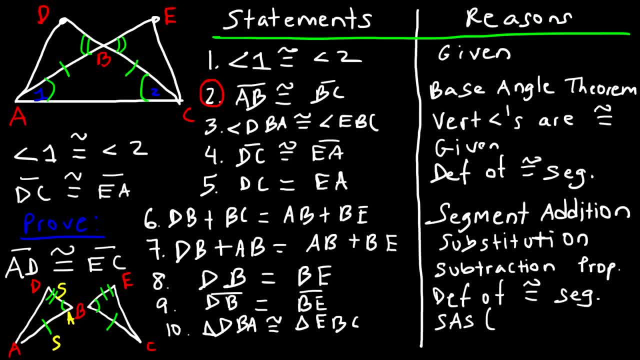 number two, number three for the vertical angles and also number nine. So it's two, three, nine. Now, finally, we could say that in statement eleven, what we're trying to prove AD, is congruent to EC. 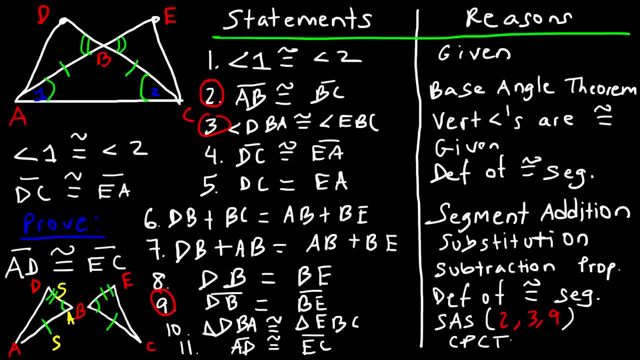 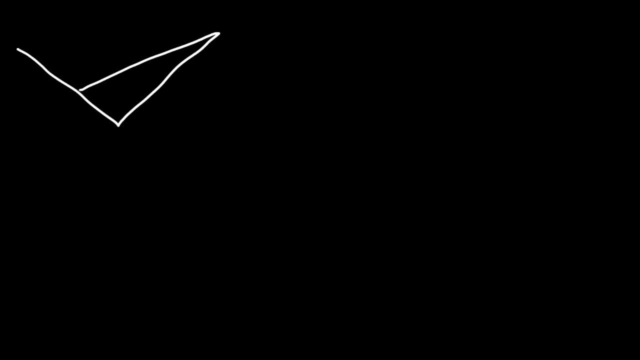 And so that's based on CPCTC. Now let's consider our final example. So let's say, this is point A, B, D and E, And in this problem we're given that BD is congruent. 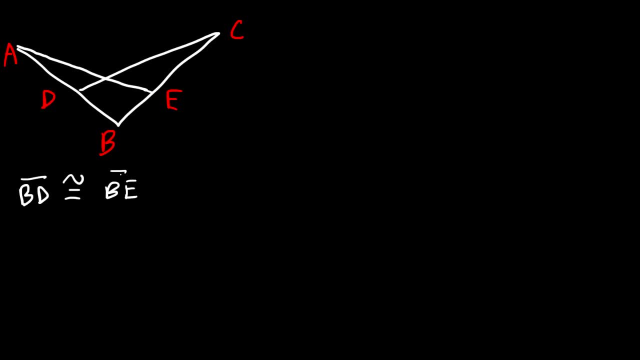 to BE And also that AO- I mean not AO, but AD- is congruent to CE. Prove that AE is congruent to DC. So go ahead and try this problem. So let's start with number one. 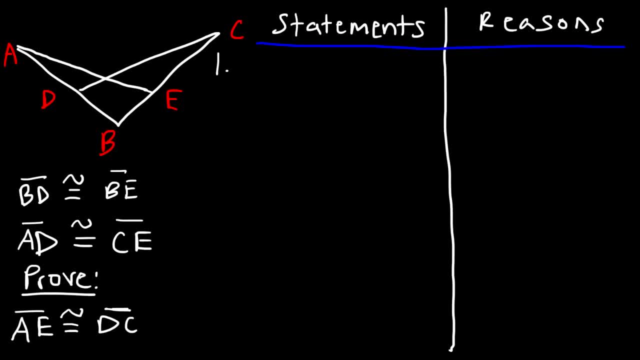 Now we know that BD and BE are congruent, So let's write that And that's given Now, in order to prove that AE is congruent to DC. what triangles do we need to prove must be congruent? 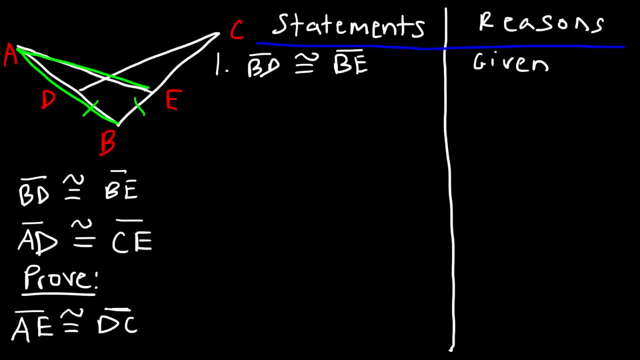 So if we can prove that triangle BE or BAE is congruent to BCD, then we can show that AE is congruent to DC. So just keep that in mind. Now let's write the second given: AD is congruent. 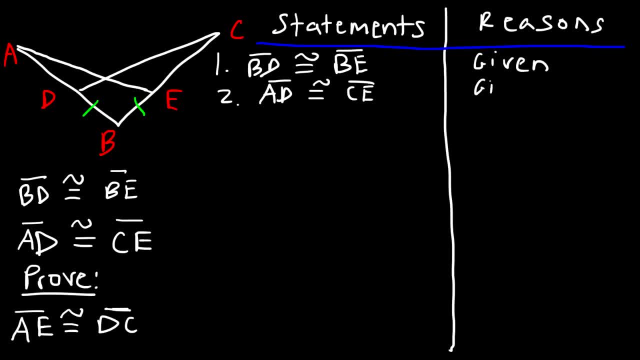 to CE And I'm going to write what we need to prove on top so I can make some space on this board. Now let's draw the triangles that we need to prove that are congruent. So this is triangle ABE. 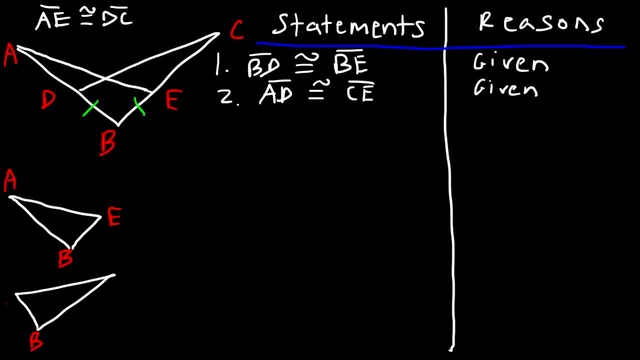 And we need to prove that it's the same with BDC. Now we know that BE is congruent to BD. So that's the first part, That's finished. And in the second sentence we know that AD is congruent to. 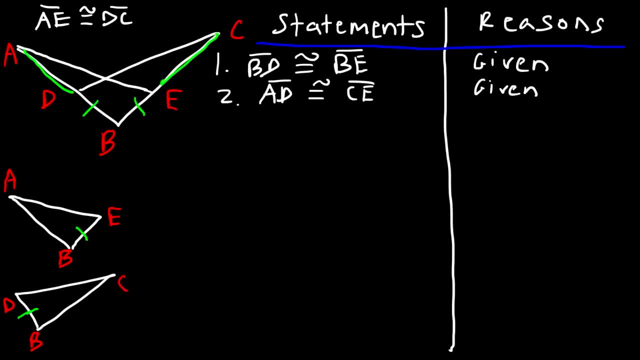 CE. So if we can add these two segments and combine those two segments, then we can show that this side, AB, is congruent to BC. So let's do that. So let's change this. This is going to be. 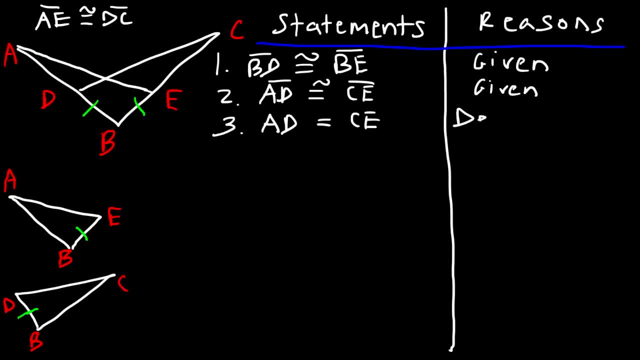 AD is equal to CE, And that's definition of congruent segments. So now what I'm going to do is I'm going to add BD to both sides of this equation. So, in step four, AD plus BD is equal to. 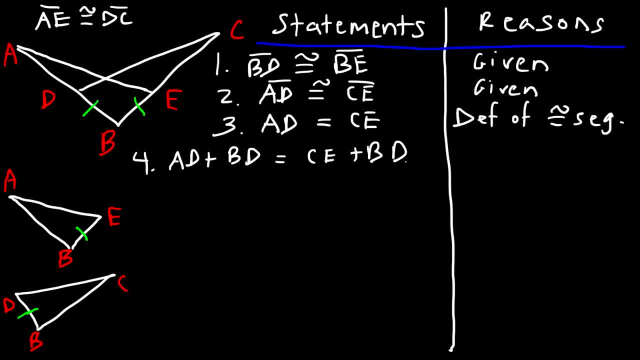 CE plus BD And that's basically the addition property, The addition property of equality. Anytime you add to both sides of the equation by a constant value, that's the addition property. Now, in step five, notice that BD and BE are the same. 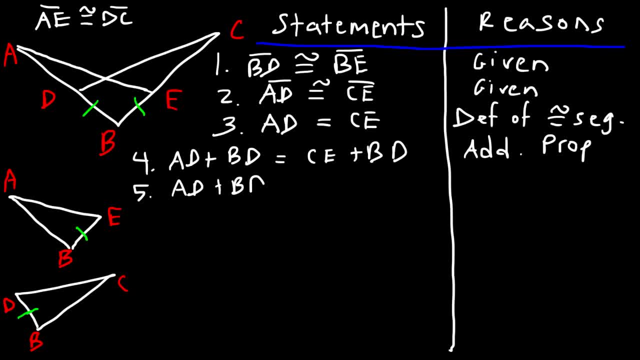 So on the right side I'm going to replace BD with BE. So I'm substituting BD with BE. So that's the substitution property. Now in step six we can add AD and BD. So this is AD. 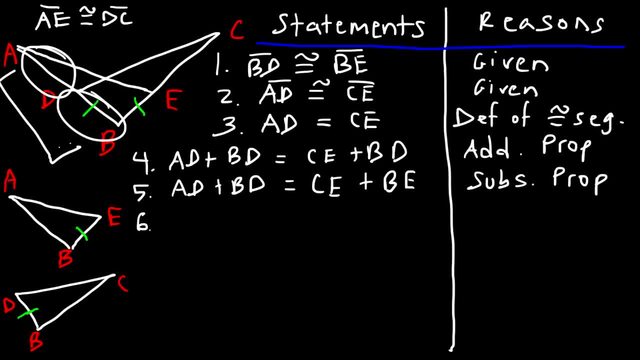 and this is BD. combined That is equal to segment AB. So AD plus BD is AB And CE plus BE is basically BC. So AB is equal to BC Based on segment addition. Now in step seven we can say that segment. 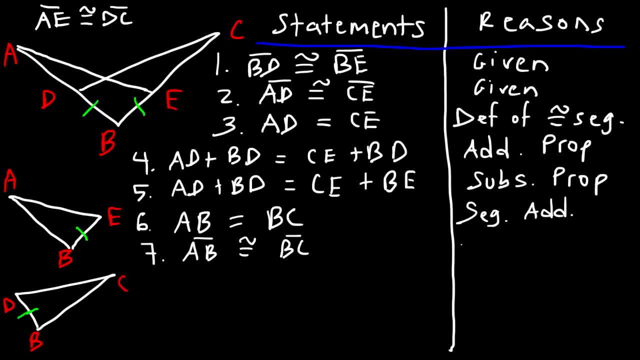 AB is congruent to segment BC And that's definition of congruent segments. So now we can mark that on the triangle. So this is AB and this is BC. They're congruent. Now notice that these two triangles share a common 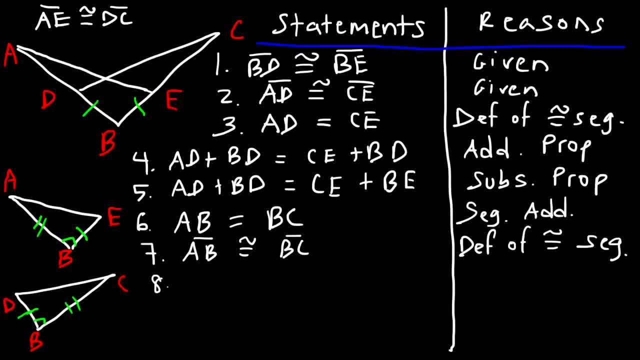 angle, That is angle B. So in step eight we can say that angle ABE is congruent to angle CBD. So triangle ABE is congruent to angle CBD And we can use the reflexive property for that. 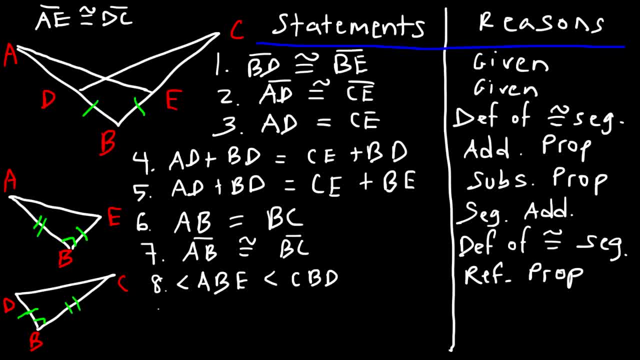 Because it's a common angle. Now, in step nine, we can now say that the two triangles are congruent. So triangle ABE is congruent to triangle CBD And this is based on the side angle, side postulate. 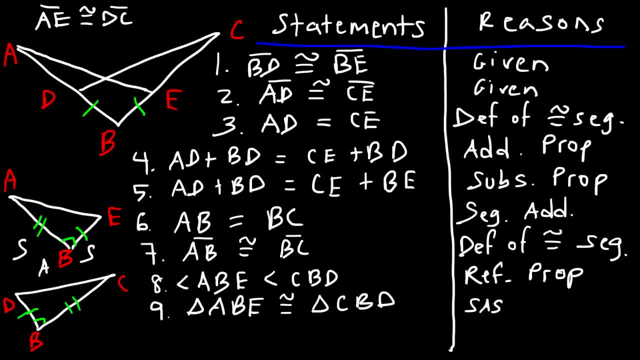 So let's start with this one. Actually, no wait, Let's start with this one. So that's based on statement one. BD is equal to BE, And then we have the angle, which is based on statement eight. 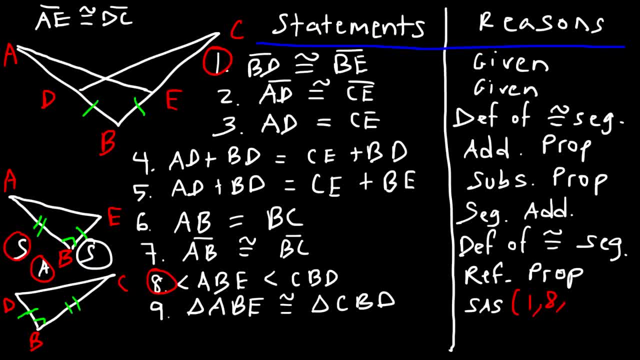 And then the third side, or rather the other side. That's based on statement seven. So, And for step ten, we can say that segment AE is congruent to segment DC, Because corresponding parts of congruent triangles are congruent. 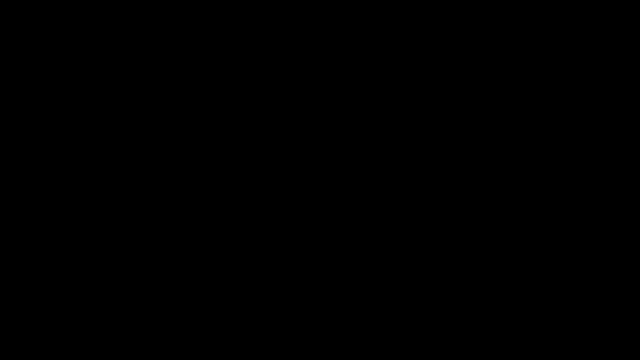 CPCTC, And that's it.